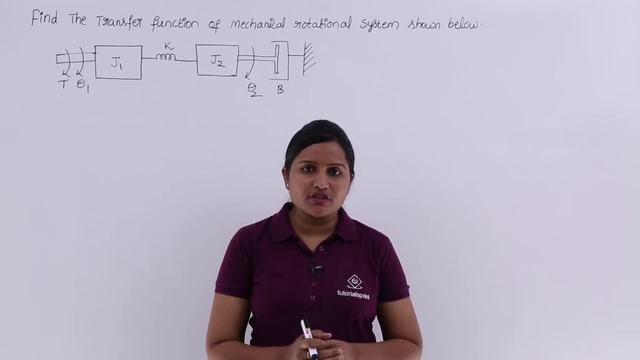 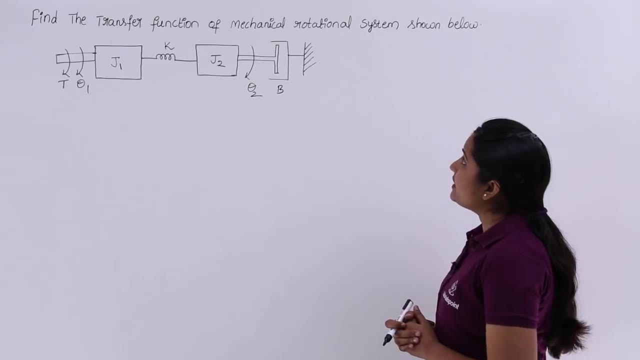 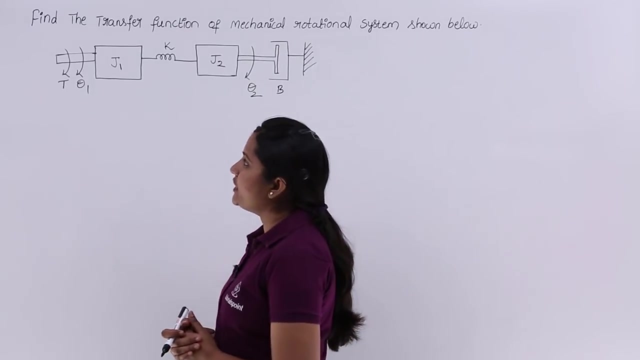 In this video we are going to discuss the transfer function of mechanical rotational system related problem. So you can see, find the transfer function of mechanical rotational system shown in figure. So this is the mechanical rotational system given. So for this we need: 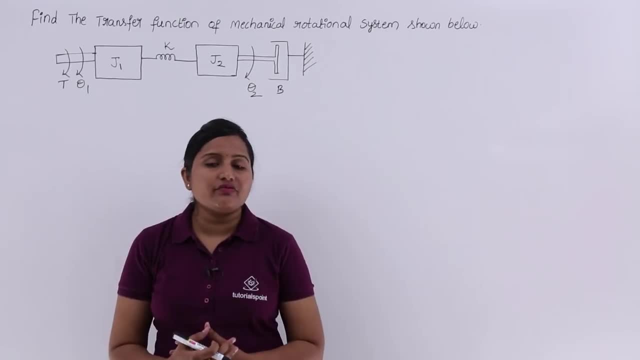 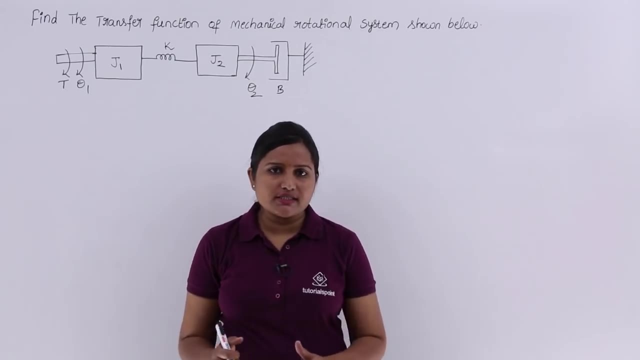 to write the transfer function. we need to get the transfer function related to this system. This is very similar to mechanical translational system. So in rotational system we will get moment of interior, j 1 in terms of mass, m 1 and remaining is same. In place of spring, you are. 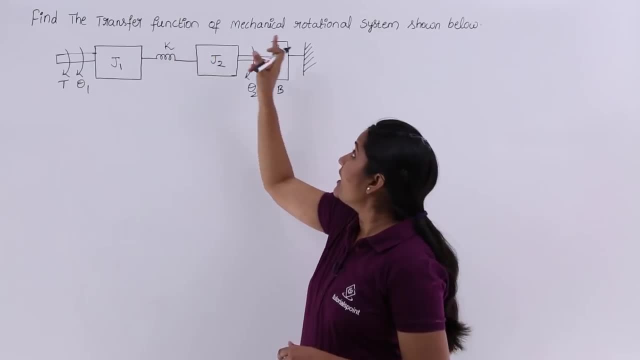 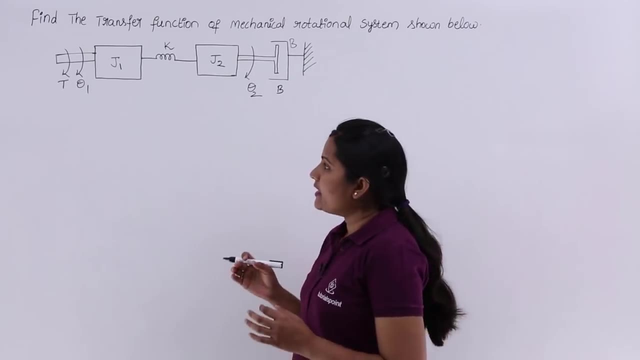 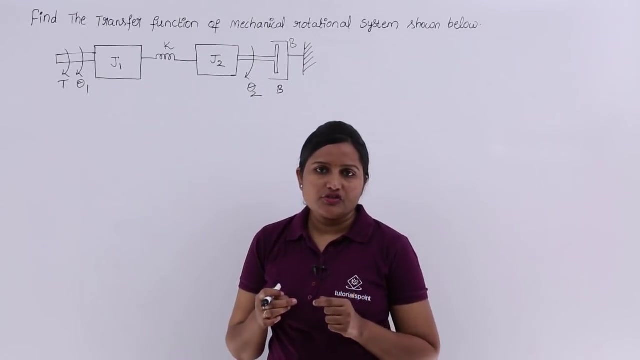 having same elasticity constant k In place of this dashpot. you are having same friction coefficient b and only we need to replace is we need to replace force with torque. So earlier we written force equations in the previous video. So we have written force equation in the previous video. 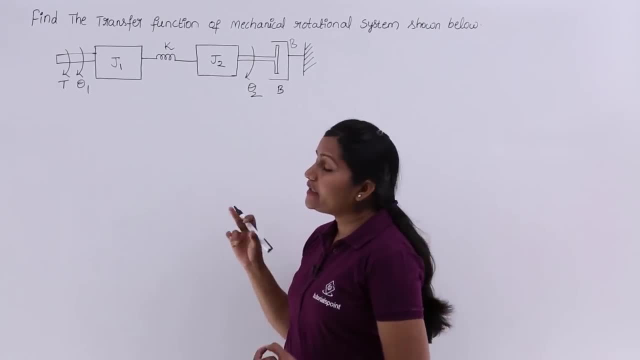 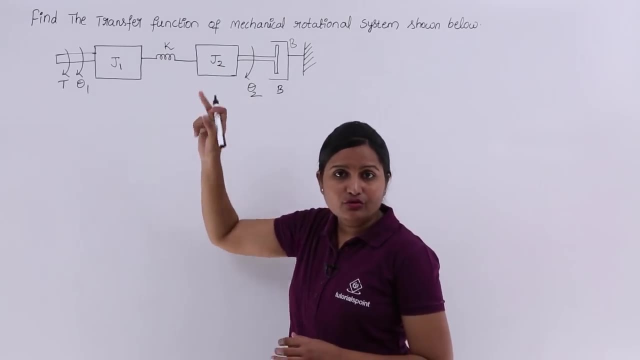 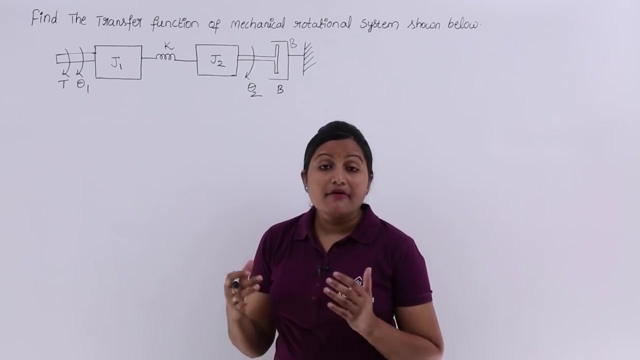 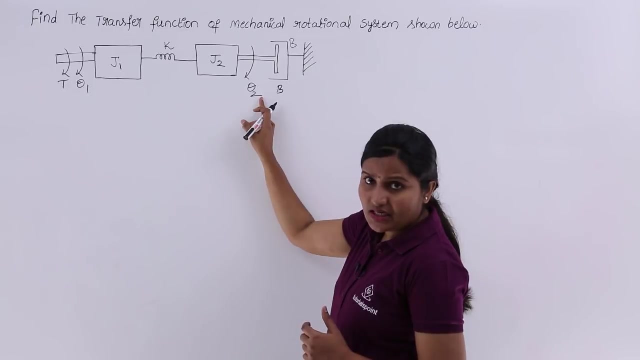 Mechanical translational system. here we need to write torque equations for each mass element, That means for j 1 and j 2. we need to draw free body diagrams from that. we need to get the torque equations from the torque equations. So we need to get So t, so this theta 2 of s by t of s. 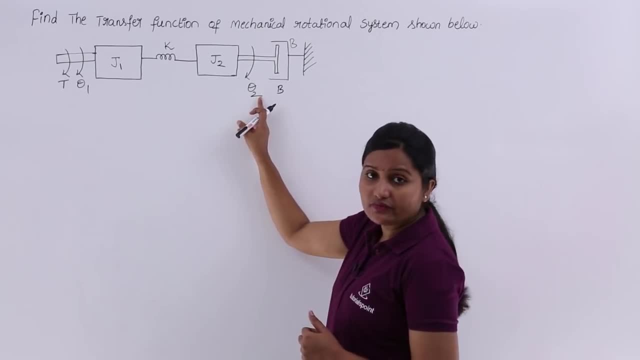 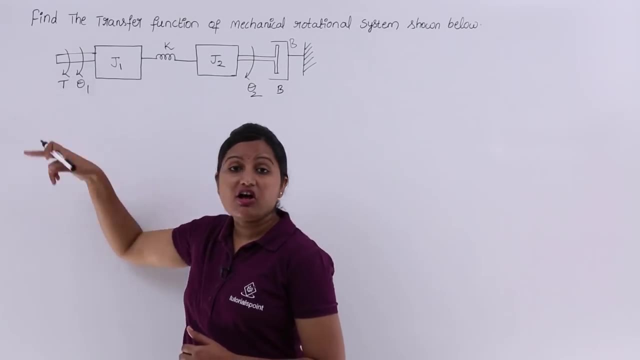 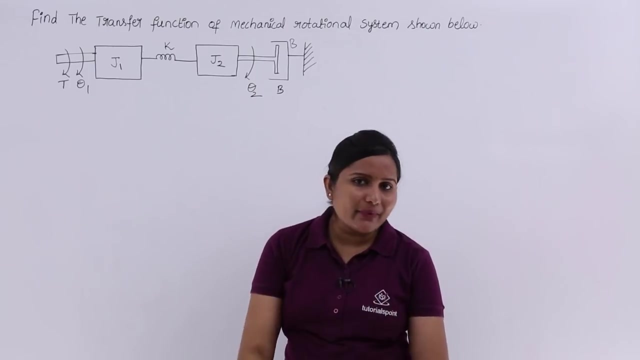 will be the transfer function here. So this theta 2 of s by t of s will be the transfer function here. Then output is in terms of displacement and input- here is a torque, input torque. So this is t, is always applied torque. If t is not there, we can say there is no applied torque for that mass. 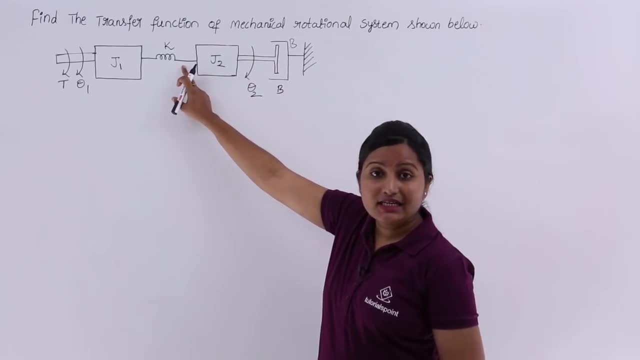 element. So for example, for this there is no external t, external torque we are not going to apply. So only torque due to that mass elements we are going to consider. So we are going to consider for this mass, but for this mass, torque due to external elements, torque due 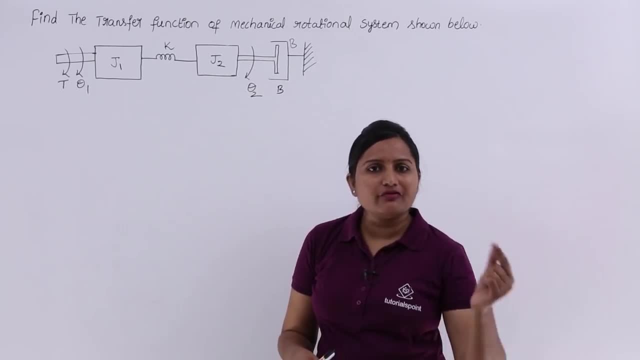 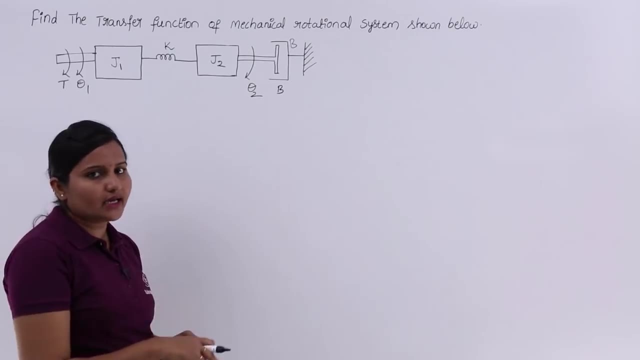 to mechanical system as well as applied torque we are going to consider. So here I am going to draw the free body diagrams similar to Mechanical translational, but here the equations are related to angular displacement, angular velocity and angular acceleration. the dark equations are like that. What I want to show is not that the force 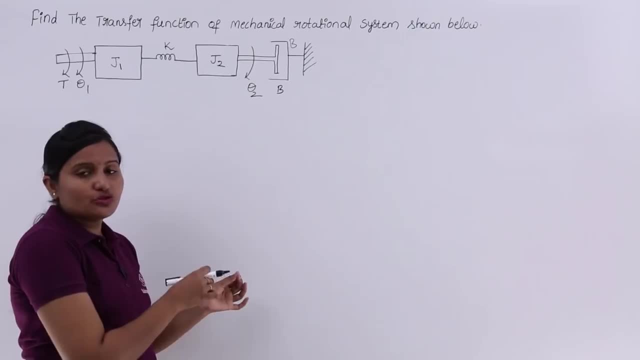 that, drawn from the present automaticzuations in the field, have no physical similar to to that. Before getting into this problem, it is better to refer that video related to mechanical rotational system and that elements. So here that video will show you how to consider the. 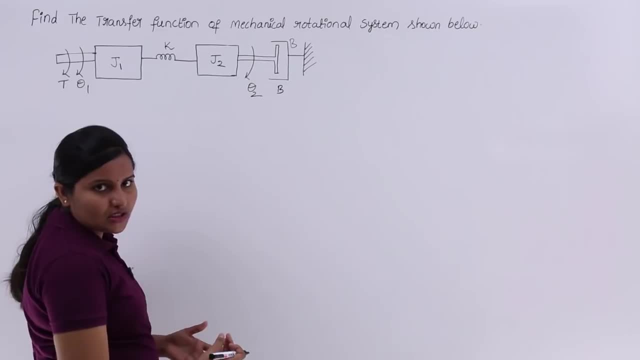 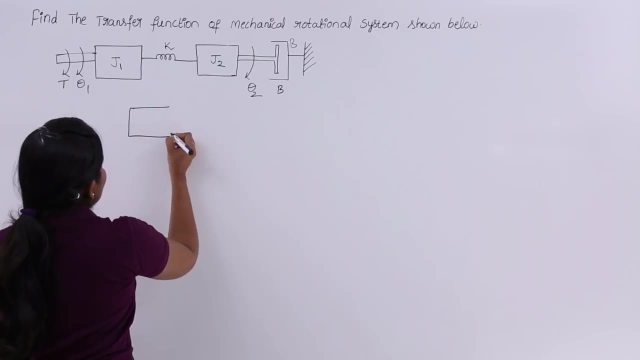 torque equations: how to write torque equations for that mechanical rotational system. So now I am going to consider my first mass J. this is my first mass J1. So this is a moment of interior. So on this. so this is displacement, theta 1 is displacement here and here an external. 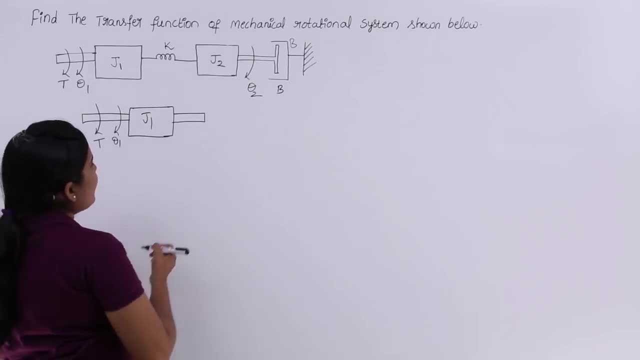 torque is acting. applied torque is T, and what are the torques on? this mass Means? the opposing torques are torque due to itself. that means T, J1. this is one torque. another torque is due to this spring. you can see this spring is attached to J1. So this 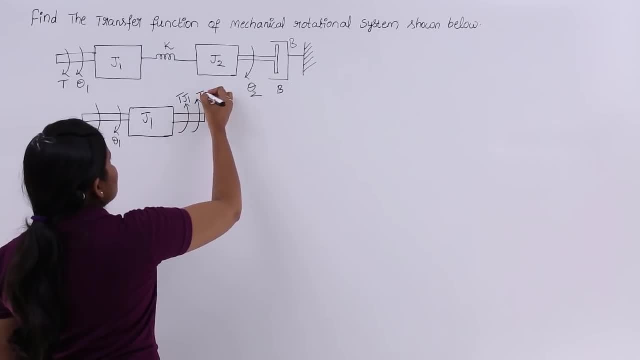 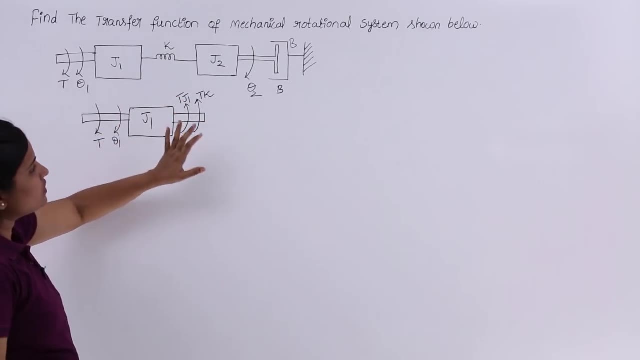 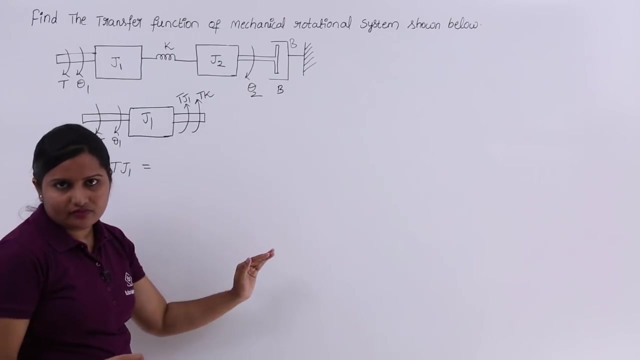 spring. due to this spring, you are having Tk and no other torques are there. why? because there is no dash spot here. So that is why Only dash spot, Only these two torques are acting. Now, how we can write T J1? T J1 is similar to F M1. 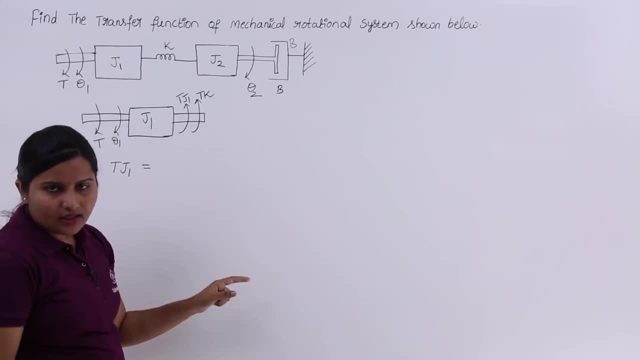 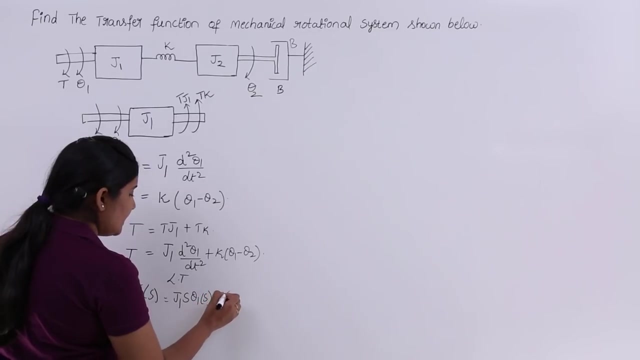 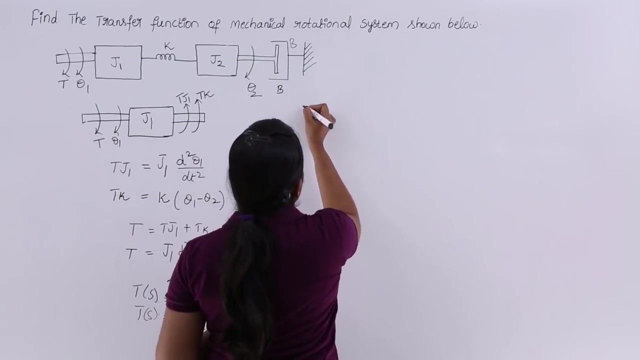 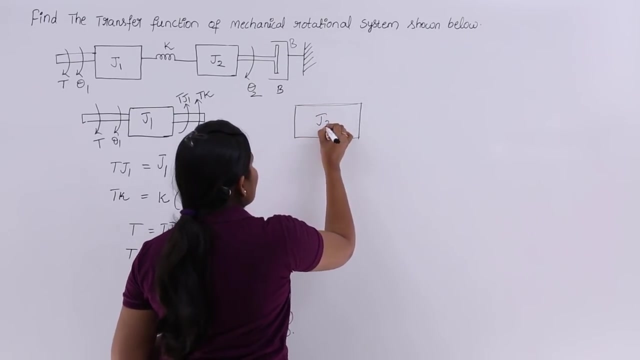 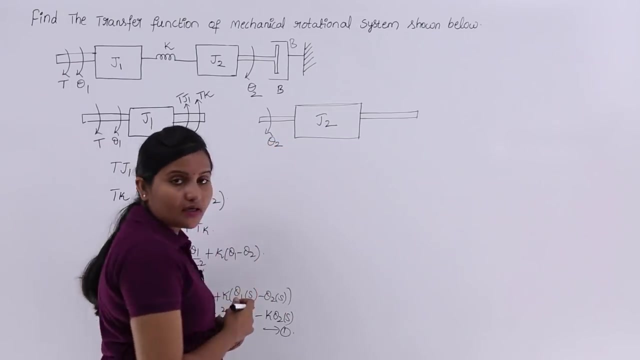 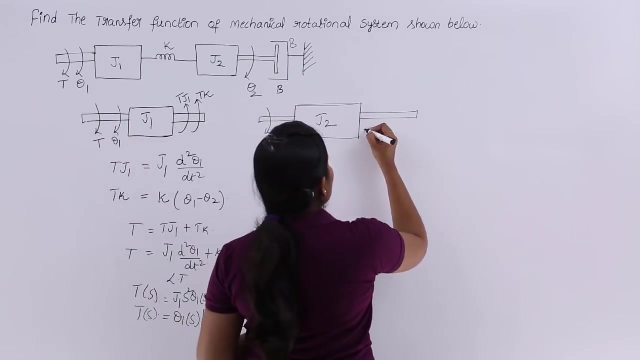 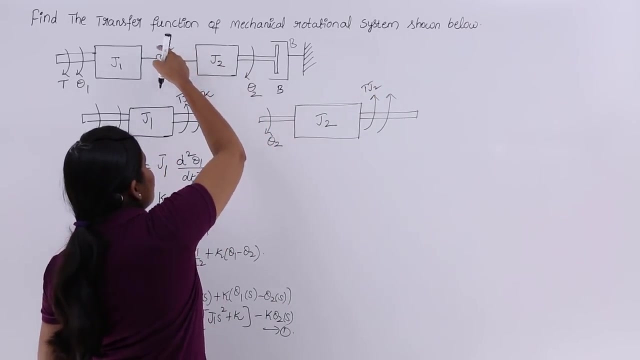 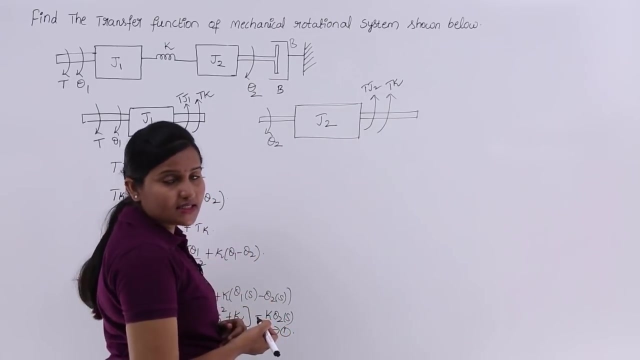 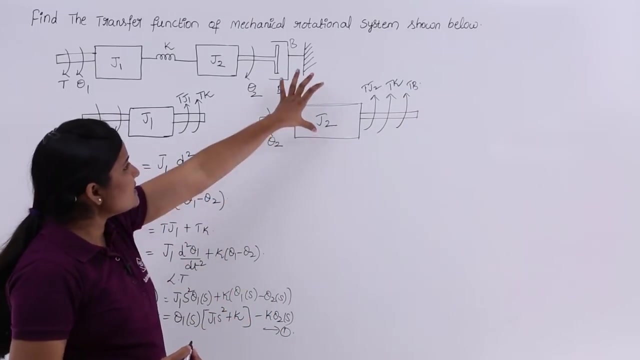 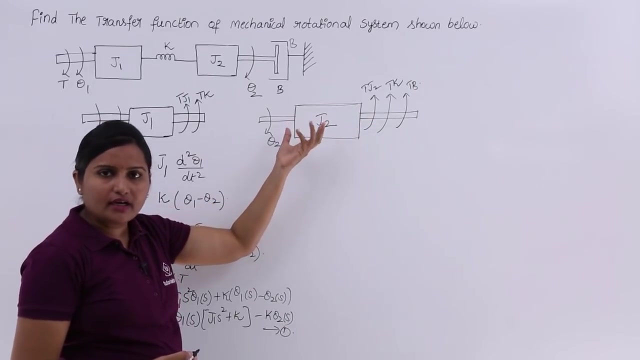 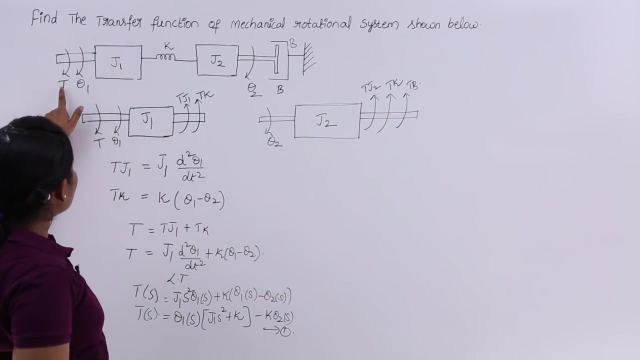 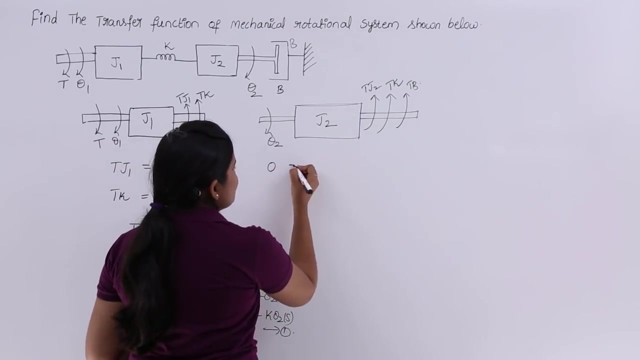 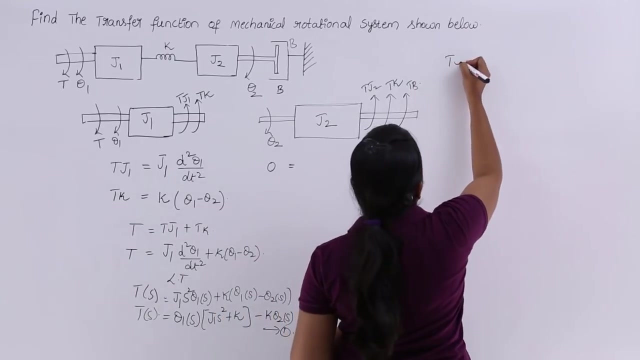 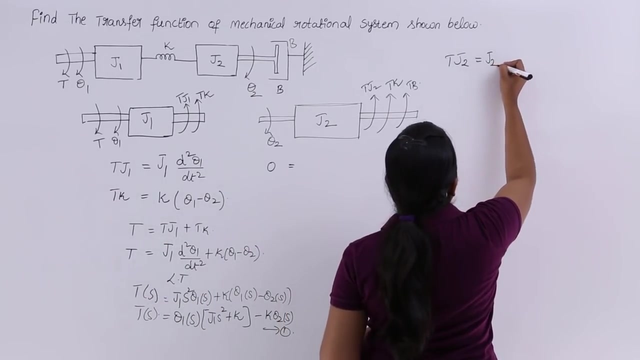 force due to mass. this is also torque due to mass, If you are considering force due to mass in rotational translational system or torque due to moment of interior in rotational system. So here the displacement is theta 2.. So that is why d square, theta 2 by g, T square. 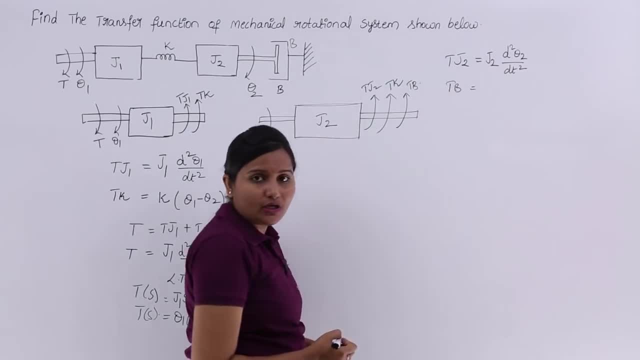 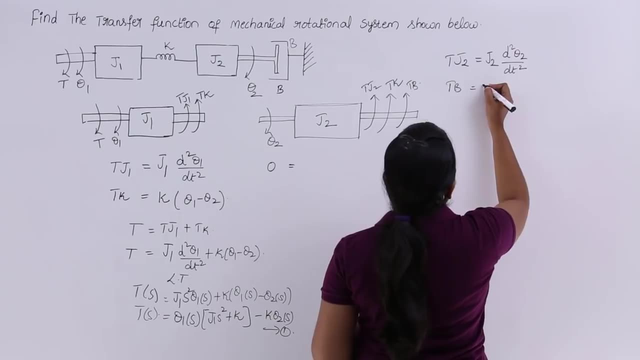 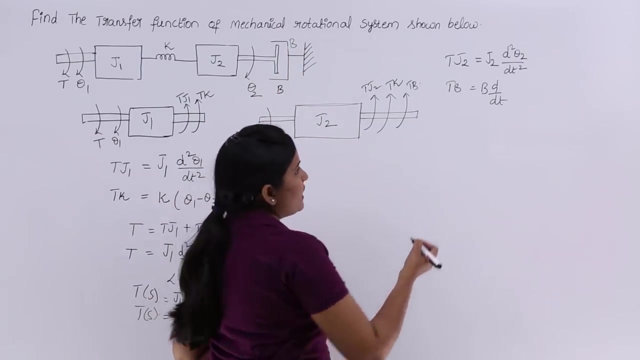 and T b torque due to dash spot. torque due to dash spot will come by using angular velocity. So here b into so d by g T of here this b is fixed So you can take d theta 2 by g T. 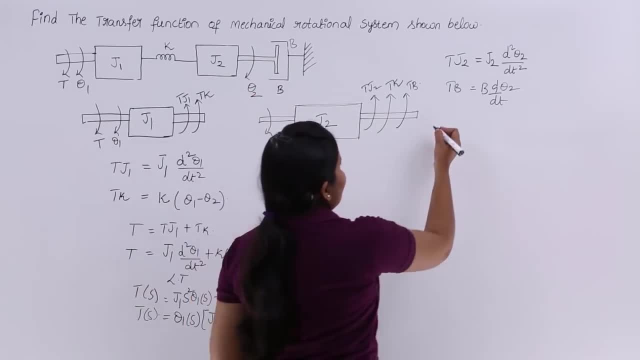 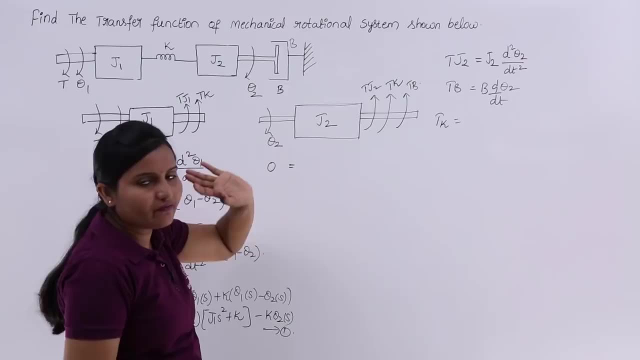 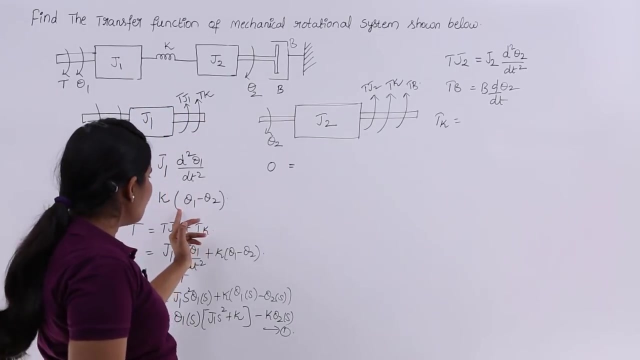 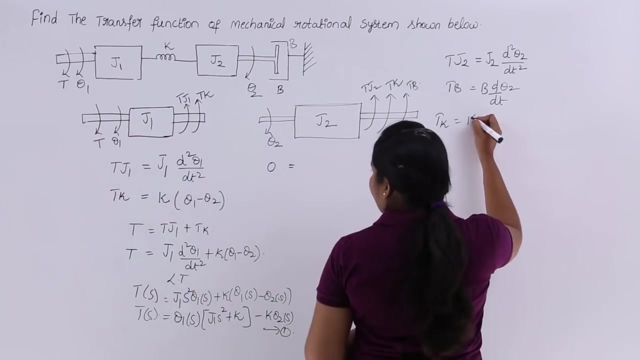 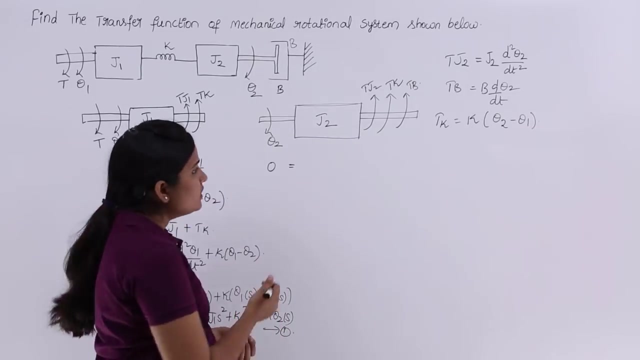 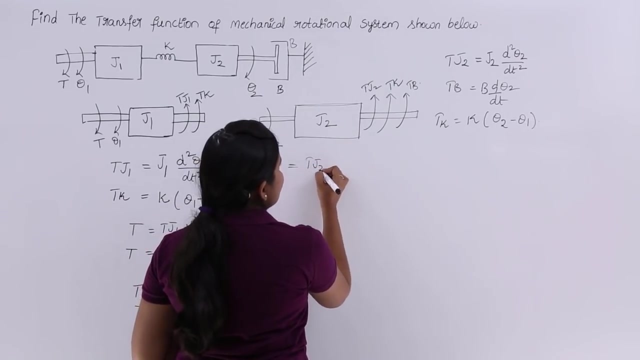 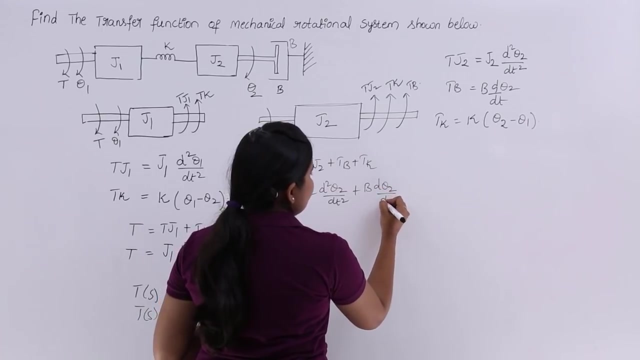 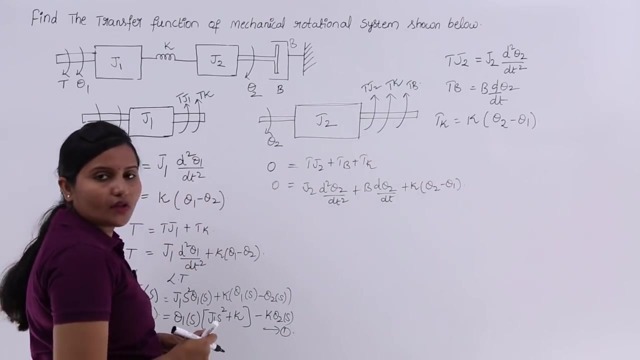 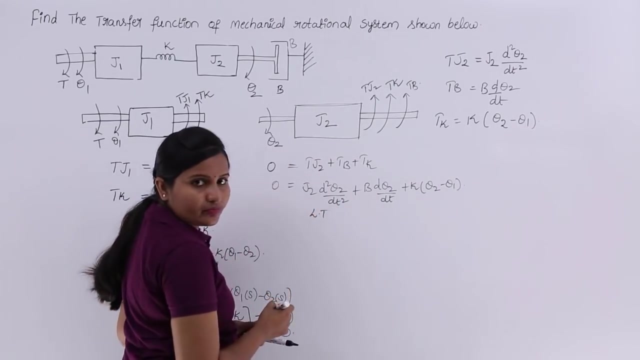 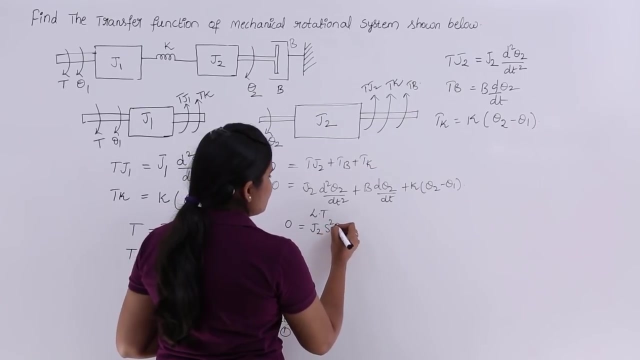 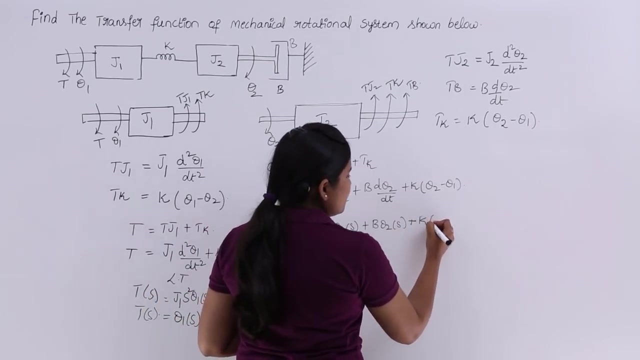 Sample time: theta 2 minus theta 1. Now here you can see. here also I am going to consider the Laplace transform, Laplace transform on both sides. So 0 is equivalent to J2 s square theta 2 of S plus b, into theta 2 of S plus K, into theta 2 of S minus theta 1 of. 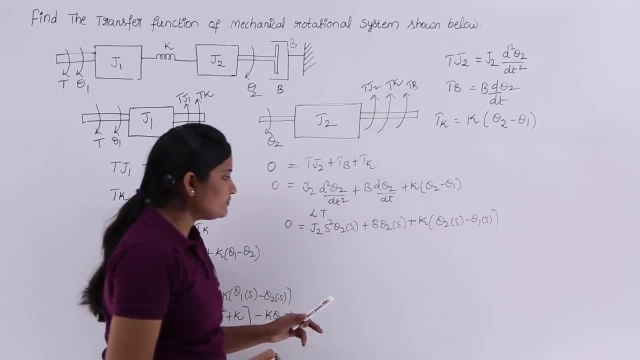 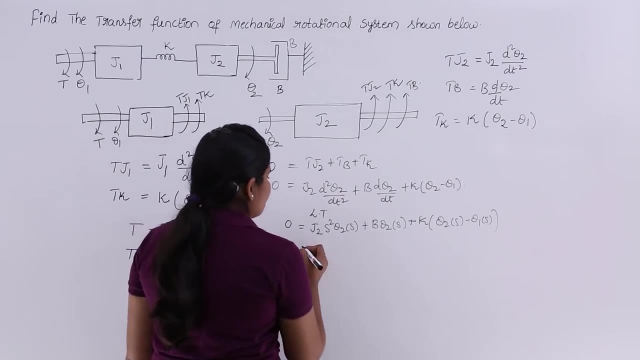 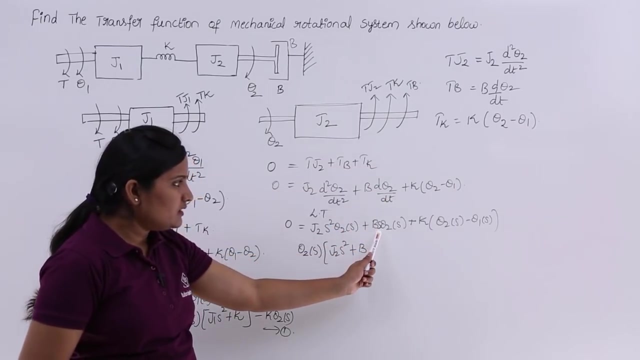 S of S. So in this equation I am going to take common of theta 2 of S, So theta 2 of S into J 2 S square plus B. So here you forgotten to write S. Why? because d theta 2 by dt. if 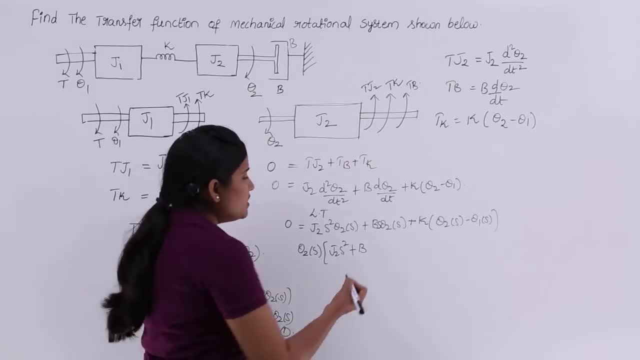 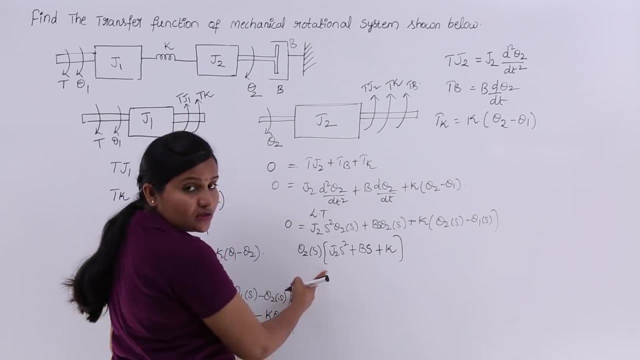 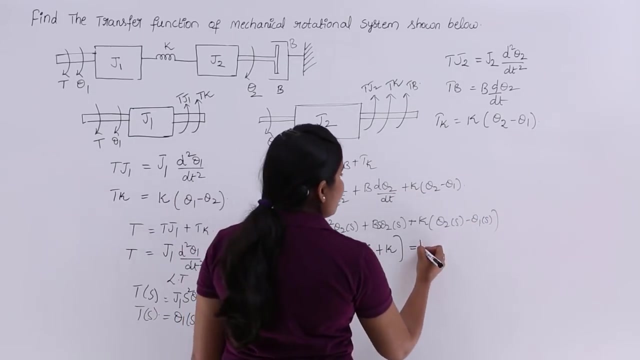 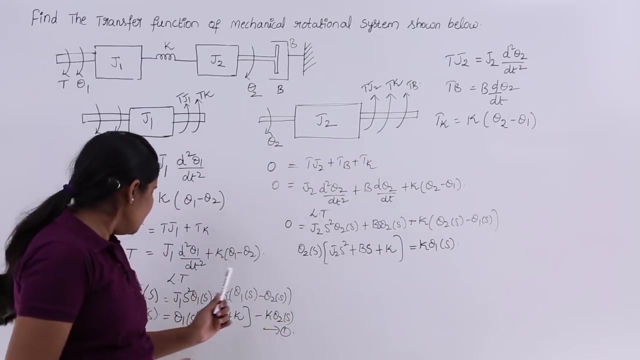 you consider Laplace transform, you are going to get S here. So B S plus K. So this is theta 2. common factor is equal into. I am sending this remaining theta 1 of S minus theta 1 of S term to this side, K into theta 1 of S. So by this equation we can write the equation. 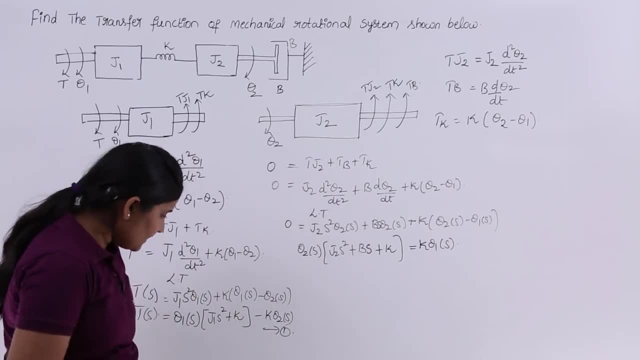 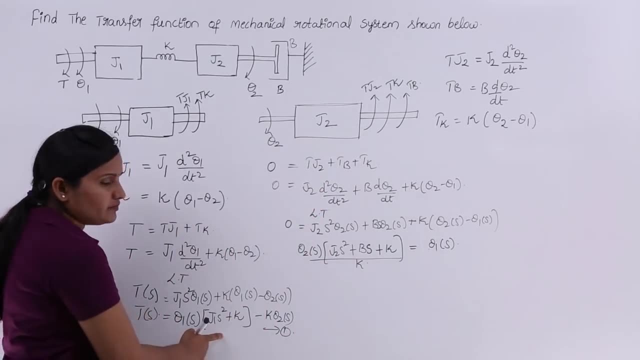 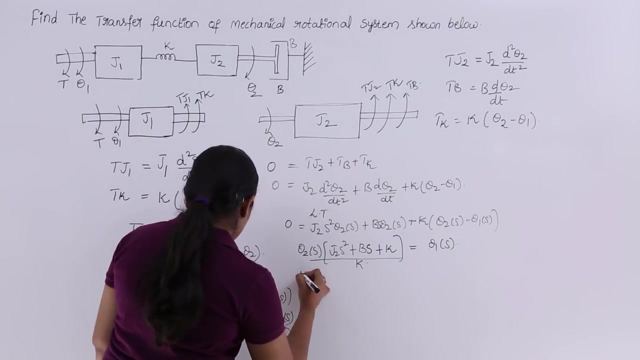 for theta 1 of S. by this equation, Theta 1 of S is equal into divided by K. I am substituting in this equation. I am substituting that theta 1 of S here. So here I am going to get. So T of S is equal into in place. 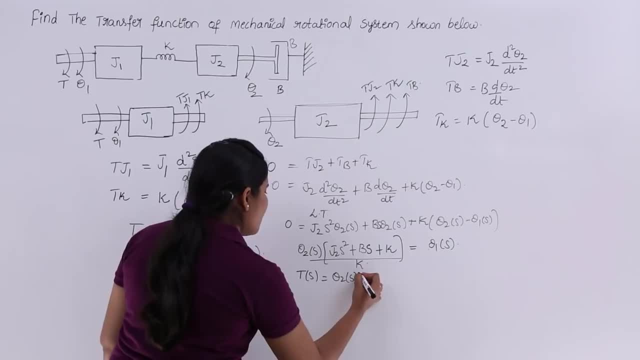 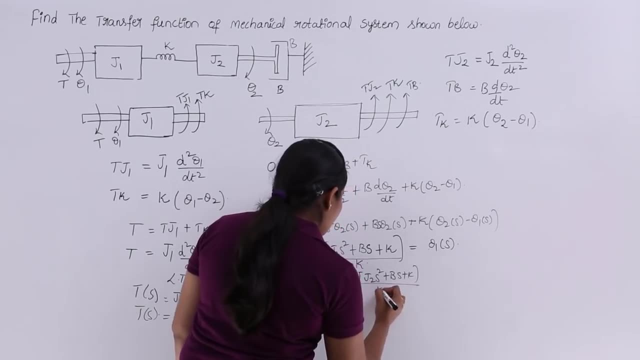 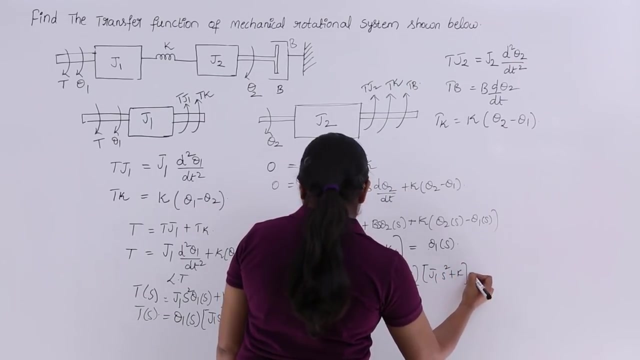 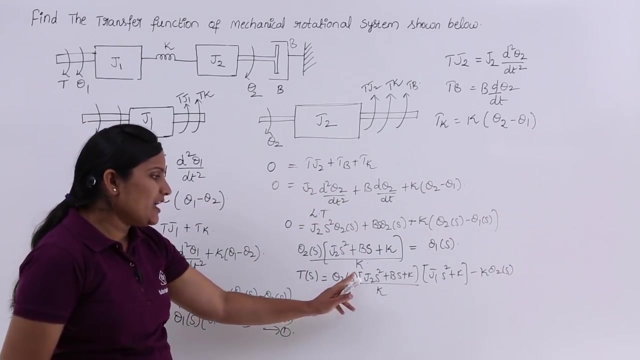 of theta 1 of S. I can write theta 2 of S- J 2 S square plus B S plus K, divided by K, divided by K, So into J 1 S square plus K minus K, theta 2 of S. So I want to take common of theta 2 of S. 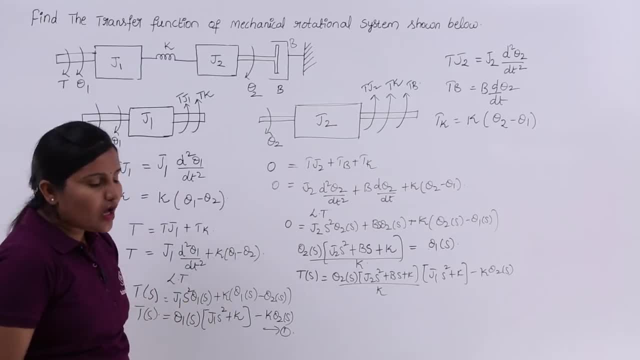 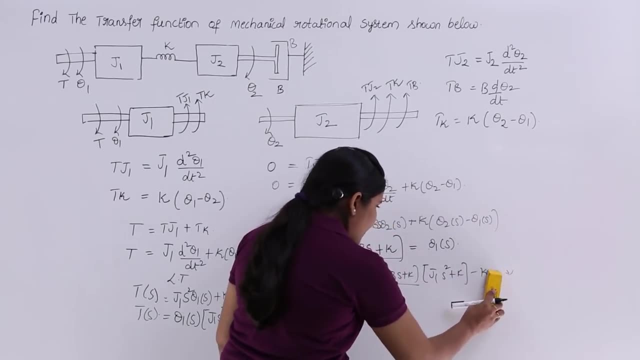 For that I require common denominator. So I am going to cross multiply this K. So now, if I want to cross multiply this K, So I am going to get K square like this. So I am taking the sign here: So J 2 delta uppercase, K 2, k theta 2 is equal to 0.. So X cross plus. 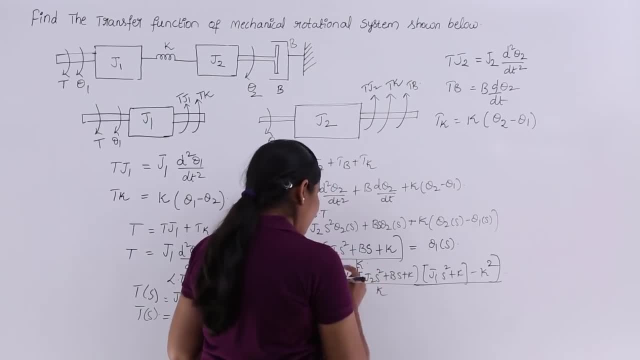 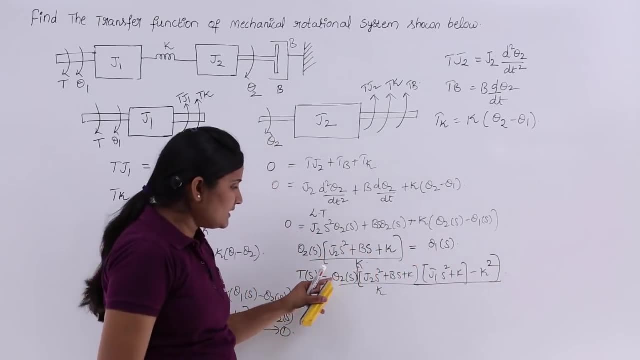 delta bar plus one plus K, times delta 3 plus K. Now I can talking byίαςiso cross multiplied and now I can take common of this theta 2 of S. So here- previously we are having theta 2 of S- I take in common of that theta 2 of S here. 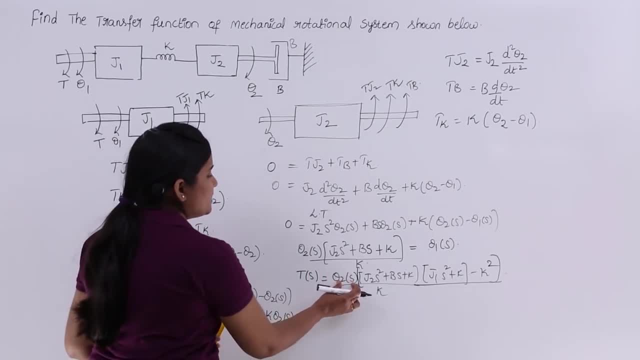 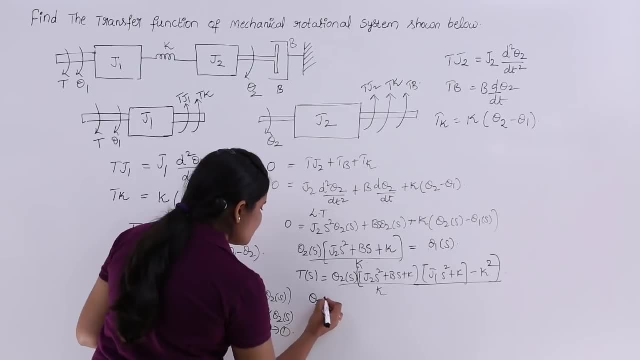 So now what we require: theta 2 of S by T of S. we require, We require transfer function of this system. That means theta 2 of S by T of S. you just send this to this side and the remainder that is taken. we have taken common denominator: The number of Y group. 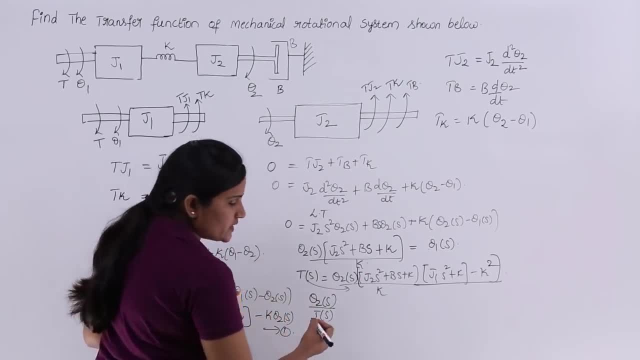 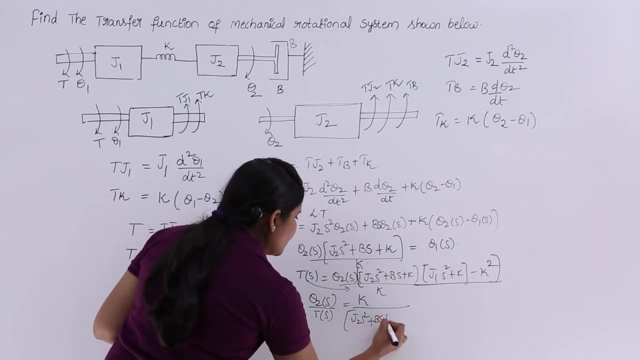 here. actually you can smaller the cube doesnot matter. So it can center in theta 2 of S in remaining thing to left side. So you are going to get K by J 2 s square plus B s plus K into J 1 s square plus K minus K square. This will be the transfer function of the. 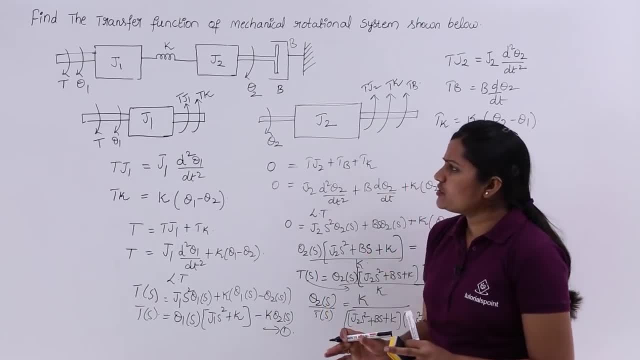 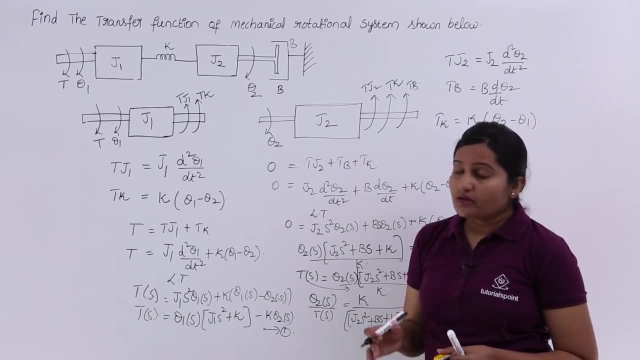 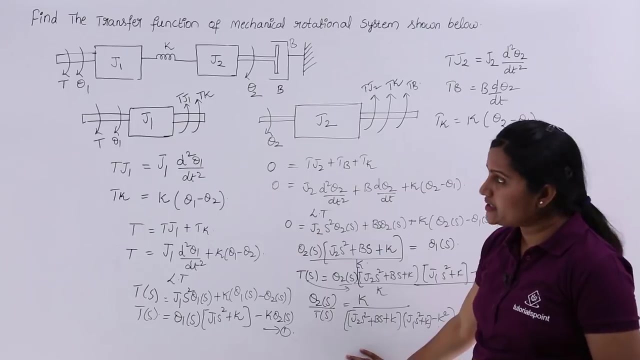 mechanical rotational system given. What we need to do is we need to do just the free body diagrams, as same as mechanical rotational system, mechanical translational system. This is mechanical rotational system, So this is the transfer function of mechanical rotational system given. So we need to write down the free body diagrams showing the total.